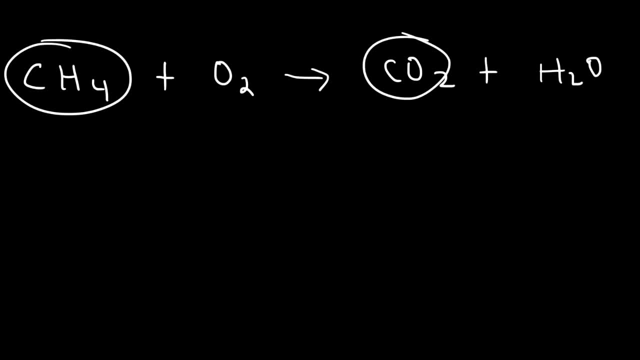 So the number of carbon atoms are balanced on both sides. We have one carbon atom on each side. Now we do have four hydrogens on the left, two on the right. So we have to put a 2 in front of water. Let's put a 1 in front of methane. 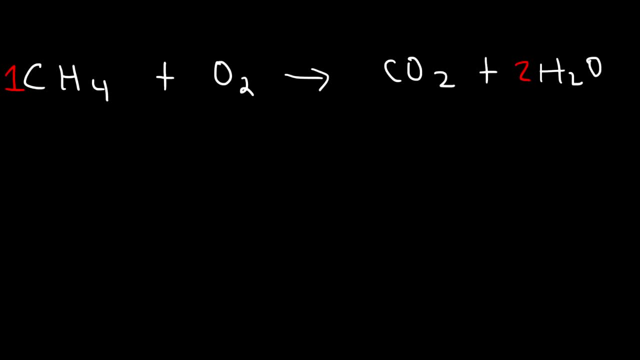 Now the last thing we need to do is balance the number of oxygen atoms. We have two oxygen atoms from the CO2 molecule and two from water, So we have a total of four oxygen atoms on the right side, So we need four on the left. therefore, we need to put a 2 in front of O2.. 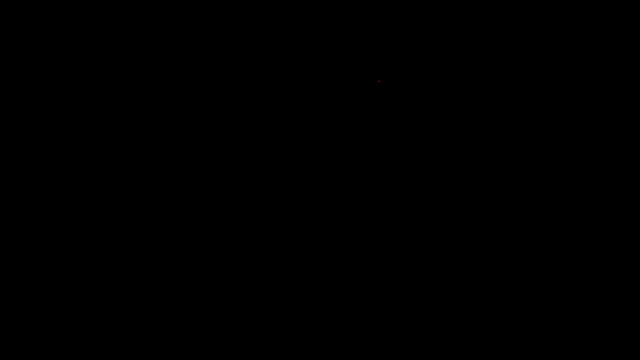 And now the reaction is balanced. So let's say, If we have C2H5OH and if we react with oxygen gas, This is another combustion reaction. so the products will be the same- CO2 and water- And you know how to balance it. so I'll leave it up to you if you want to balance it or not. 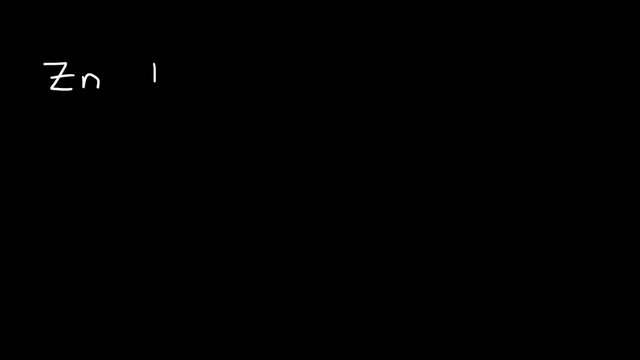 Now let's say if we react zinc with oxygen gas, What product will form in this reaction? Now, when you mix two elements together, you're going to get a combination reaction. They're going to combine and form a compound. So in this case, a compound between zinc and oxygen will have what chemical formula? 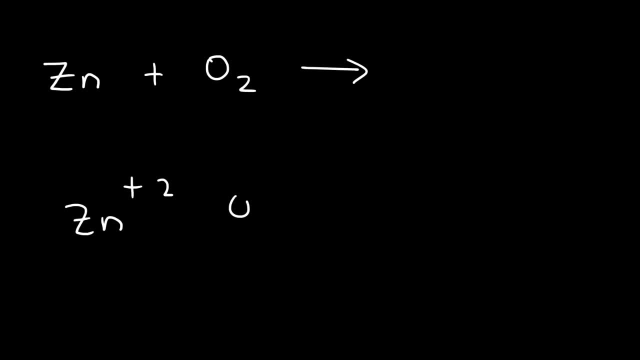 Zinc has a positive 2 charge. Oxygen has a minus 2 charge. Whenever you have two ions combining, and if they're, If they have the same charge, even though the sign is opposite, they're going to combine in a 1 to 1 ratio. 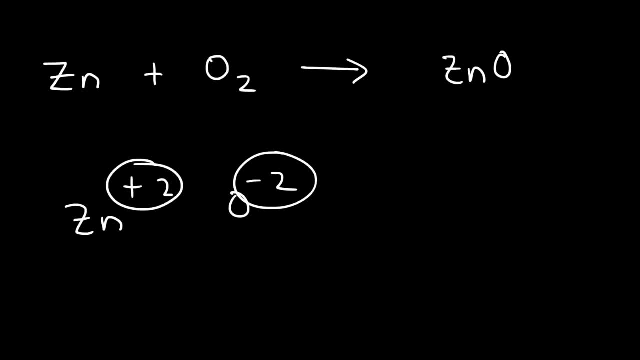 So the product for this example is zinc oxide, And if you wish to balance it, all you need to do is put a 2 in front of zinc oxide and a 2 in front of zinc, And now it's balanced. So let's say, if we want to react magnesium metal with nitrogen gas, 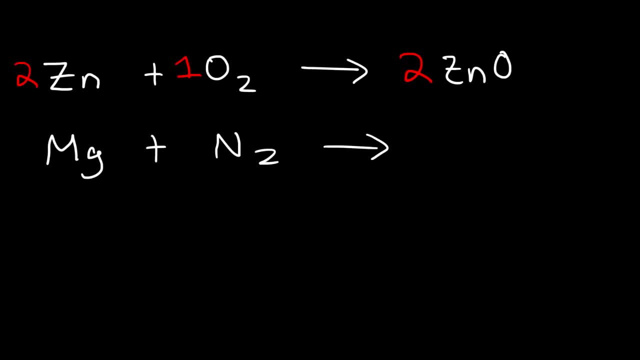 What product will form in this reaction. So we're going to get a compound composed of magnesium and nitrogen, or magnesium nitride. Magnesium has a positive 2 charge, Nitride has a minus 3 charge. So when combining these two elements, it's going to be Mg3N2.. 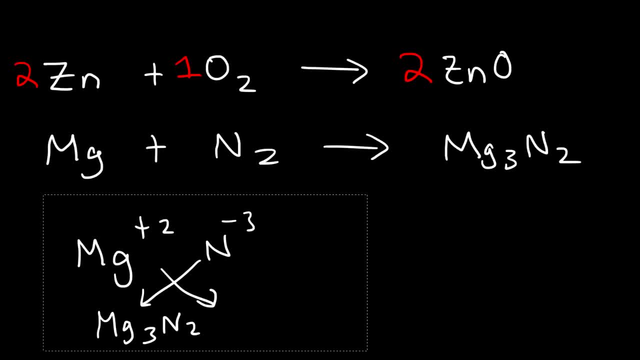 And now all we need to do is just balance it And we're done. And now all we need to do is just balance the chemical reaction. So we just need a 3 in front of Mg and a 1 in front of everything else. 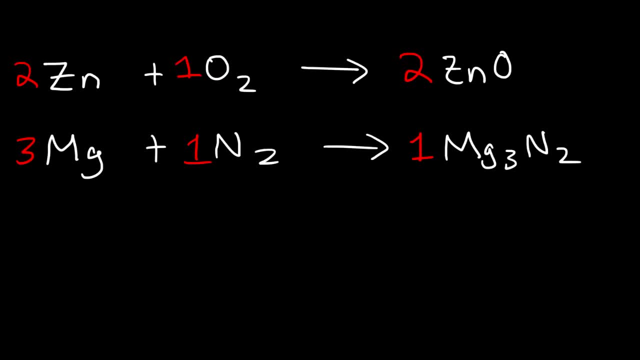 So, for the sake of practice, let's look at one more example. So let's react sodium metal with elemental sulfur. Feel free to pause the video and predict the product that will form in this reaction. So we're going to get a compound between sodium and sulfur, or sodium sulfide. 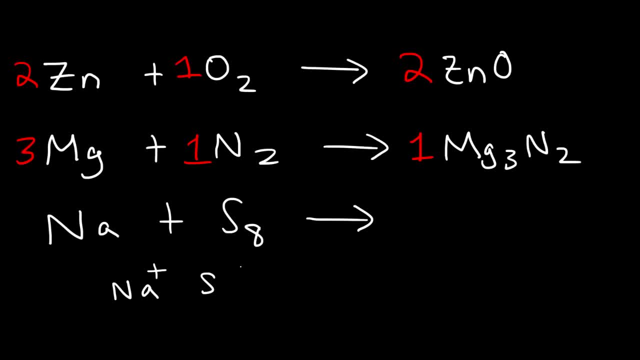 Sodium has a positive 1 charge. Sulfide has a minus 2 charge, So this is going to be Na2S1. Or simply Na2S. Now, to balance it, we need an 8 in front of Na2S. 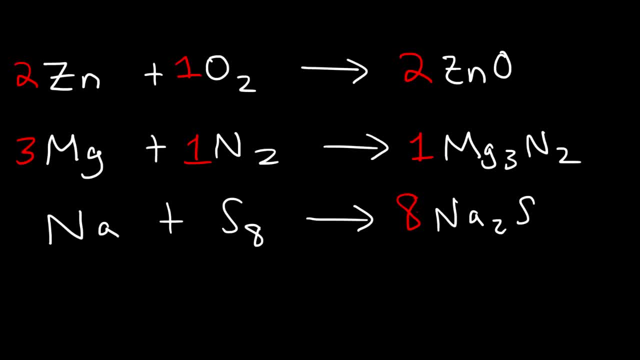 So we can have 8 sulfur atoms on both sides. Now notice that we have 16 sodium atoms on the right. 8 times 2 is 16, so we need a 16 in front of Na. And so this is how you can balance synthesis or combination reactions. 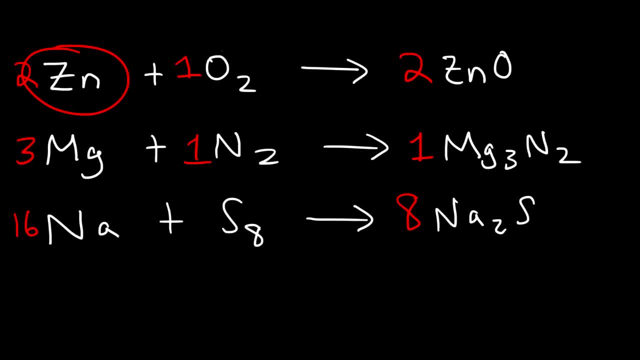 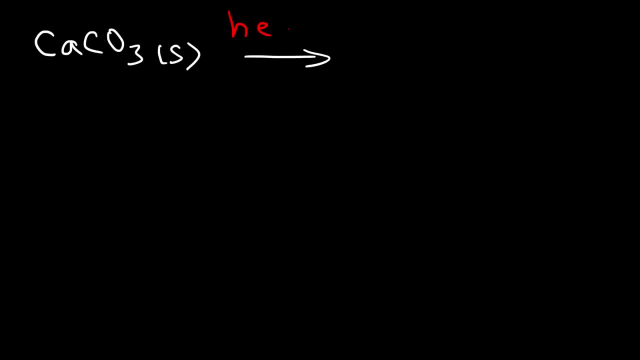 And how to predict the products If you have an element reacting with another element. Now what's going to happen if you have calcium carbonate And you subject it to heat? Anytime you heat a metal carbonate, A volatile component will escape. That volatile component is carbon dioxide gas. 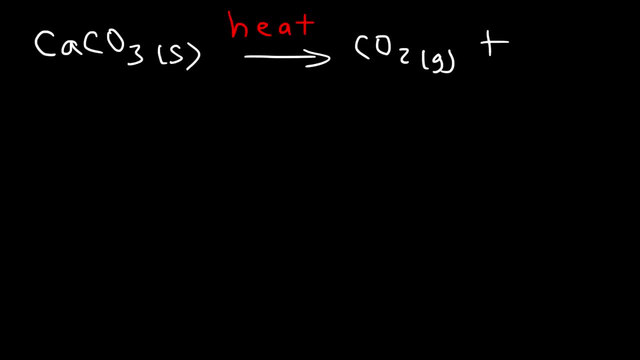 And it's going to leave behind a metal oxide, In this case, calcium oxide. So If we had magnesium carbonate And we add heat to it, CO2 will leave Producing magnesium oxide. Now the reverse is true as well. 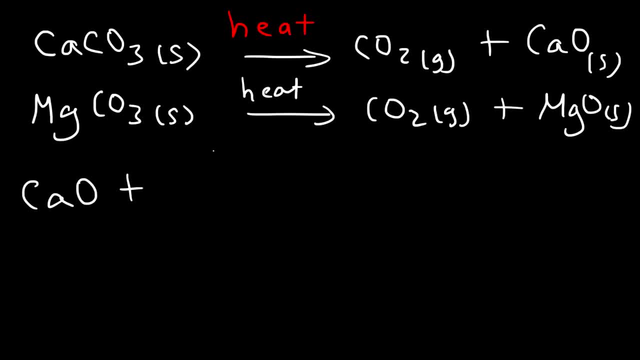 If we were to take calcium oxide And react it with carbon dioxide, This will be a synthesis reaction, But it's different from the other synthesis reactions Because we're not mixing an element with an element. We're combining two compounds And this will form calcium carbonate. 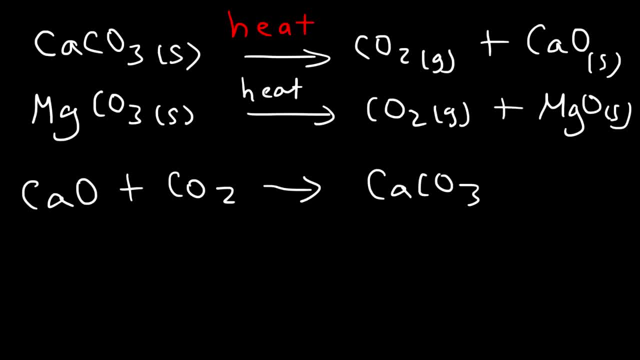 So typically The reverse of a synthesis reaction is a decomposition reaction. So if you know the decomposition products, then You know that these two combined Will just produce this If the temperature is low. Now let's say If we have a metal hydroxide. 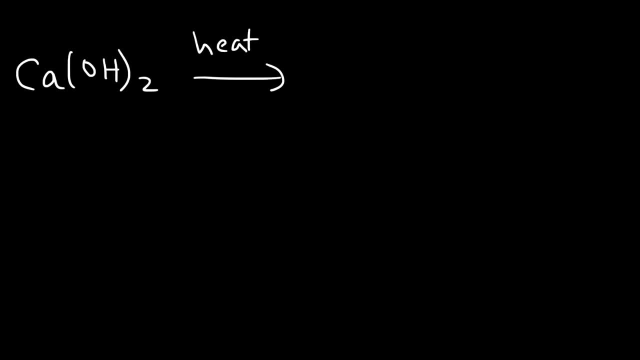 And we add heat to it. What products will be produced in this reaction? If you heat up a metal hydroxide, It's going to cause water to evaporate. Once water is removed, You're going to get the metal oxide. So let's say, if we have aluminum hydroxide, 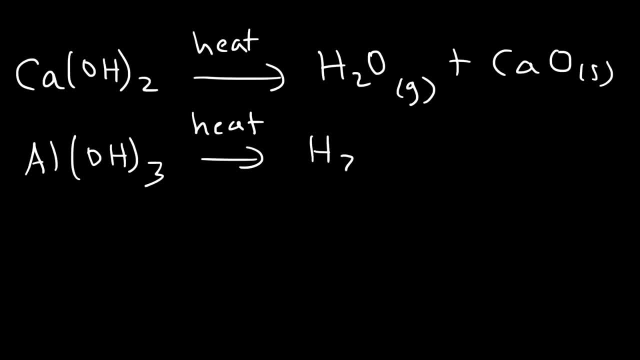 And if we add a lot of heat, Water will leave, Leaving behind aluminum oxide. Now you can balance it if you want to, But let's go ahead and balance it. Let's put a two in front of aluminum hydroxide, So now we have two aluminum atoms. 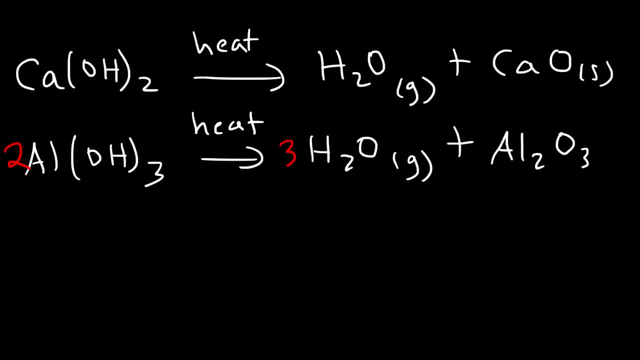 We have six oxygen atoms in total, So we need a three In front of H2O. So anytime you heat a metal hydroxide, It's going to produce water And the corresponding metal oxide. Now let's move on to single replacement reactions. 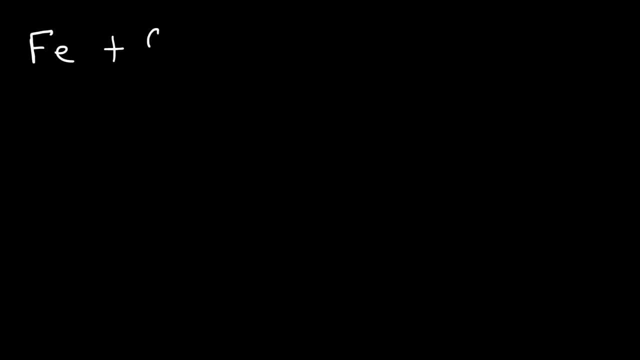 Let's say, if we react iron metal With copper chloride, What products will be formed in this reaction? So iron metal is a solid And We're mixing it with an aqueous solution of copper chloride In a single replacement reaction, The metal Fe. 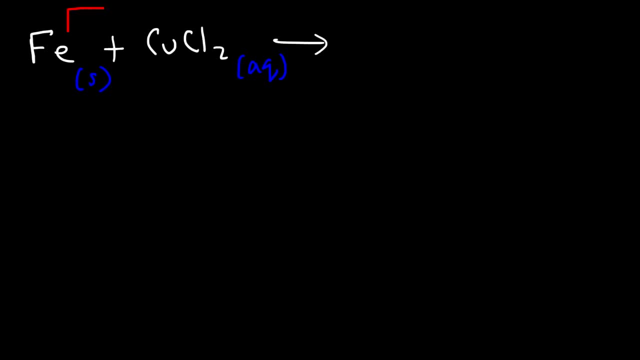 Will replace the other metal copper. So Fe is going to pair up with Cl. Fe typically has a positive charge, I mean a positive two charge. Chloride has a minus one charge, So this is going to be Fe1Cl2.. So one of the products will be FeCl2.. 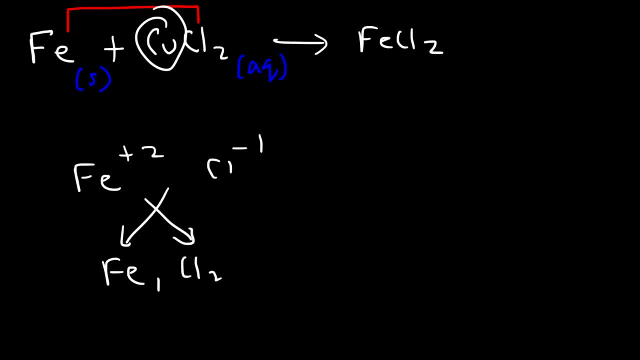 Copper is going to be displaced out of the solution As copper metal, And so that's going to be the products Of the single replacement reaction. Lets work on another example. Lets say if we have aluminum Reacting with nickel to chloride, 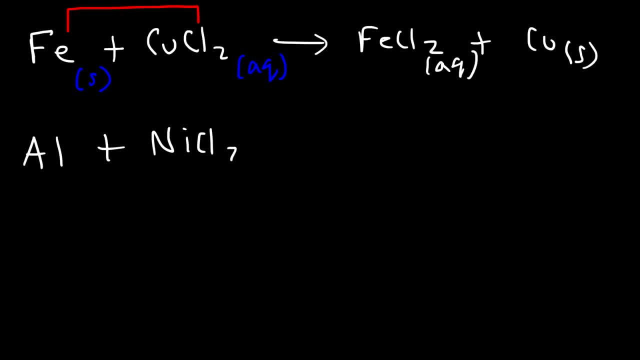 Go ahead and predict the products of this reaction. So aluminum is going to pair up with chloride. Aluminum has a positive three charge, Chloride has a minus one charge. So the chemical form of the product Will be Al1Cl3. It's going to take an associated form. 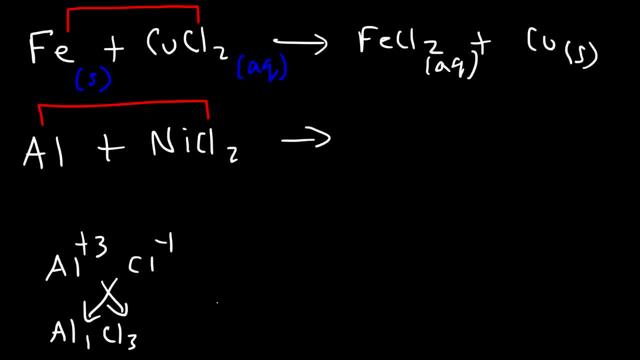 which is called L1Cl3., Cl3 or simply AlCl3, and nickel is going to be displaced out of the solution as solid nickel metal. typically, the compound, nickel chloride and aluminum chloride, is still dissolved in the solution. now what about the zinc metal reacting with hydrochloric acid? try this one. in this case, zinc is still. 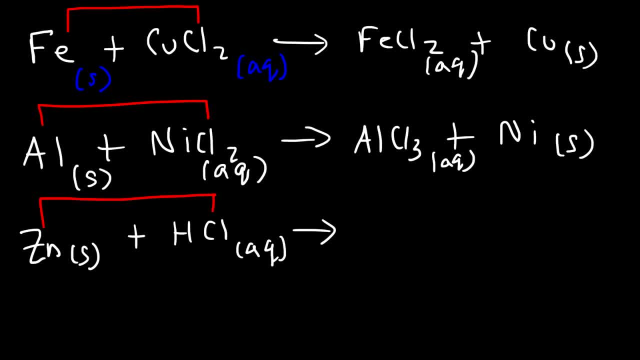 going to pair up with chlorine, the same way as aluminum paired up with the nonmetal chlorine. now let's write the formula between zinc and chlorine. zinc has a positive 2 charge, chloride has a minus 1 charge, so it's gonna be Zn1- Cl2. 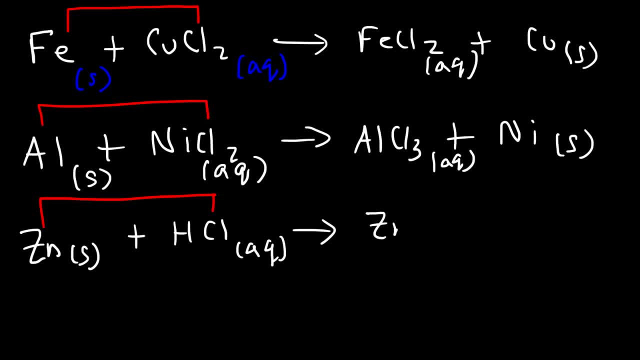 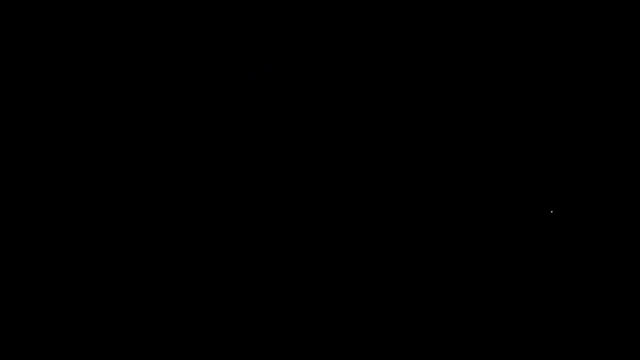 zinc is going to displace hydrogen out of the solution and so it's going to be elemental hydrogen which exists as a gas. so whenever you have an active metal and you react it with an acid, hydrogen gas will be produced. now, let's say, if we have a nonmetal like chlorine gas, reacting with an aqueous solution of 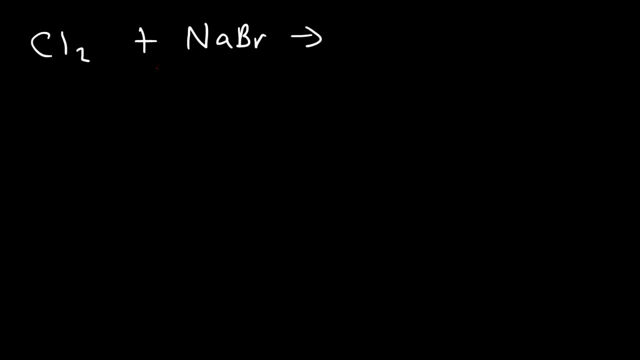 sodium bromide. what's going to be the products of this reaction? in this case, zinc is going to displace hydrogen out of the solution, so that it's going to be case Chlorine, the non-metal, is going to pair up with sodium, a metal ion, and chlorine is going. 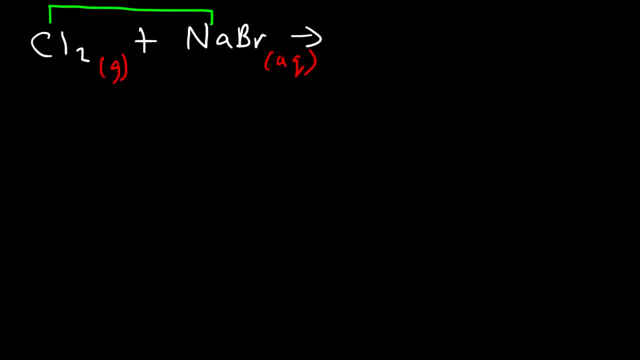 to displace the other halogen bromine out of the solution. So when chlorine pairs up with sodium, it's going to be a one-to-one ratio, It's going to be Na1Cl1, or simply NaCl and bromine is going. 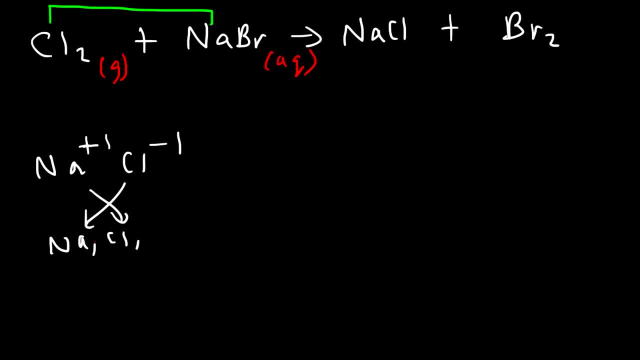 to be displaced out of the solution as diatomic bromine, which is a liquid at room temperature. So this is going to be the reaction. If you want to balance it, just put a 2 in front of NaBr and NaCl. 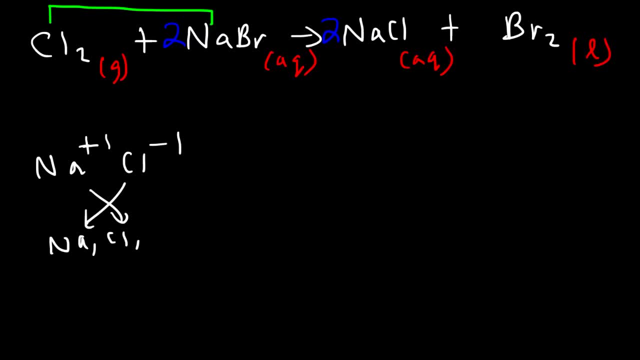 So whenever you have like a halogen reacting with an aqueous solution, typically the halogen will displace the other halogen out of the solution. So let me give you another example of this type of problem. So let's use bromine and sodium. iodide Bromine is going to pair up with sodium, producing sodium. 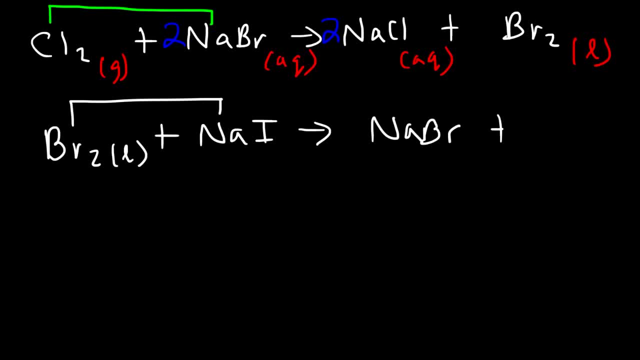 bromide and it's going to displace iodide out of the solution, And iodide is a solid. I mean iodine as a pure element And the compound is iodide, but as a pure element it's going to displace iodide out of the solution. 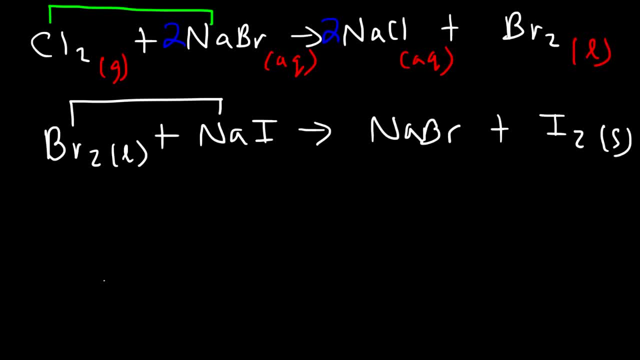 So, as you can see, the reaction is very similar. To balance it, it's going to be the same. So now you know how to predict the products of a single replacement reaction. Now let's move on to a double replacement reaction. Let's say if we have silver nitrate reacting with sodium iodide. 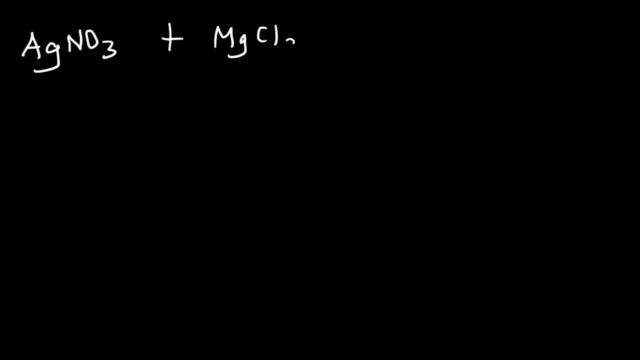 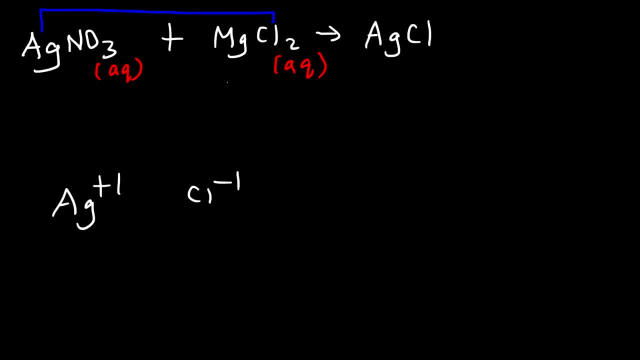 So this is going to be a double replacement reaction And then magnesium is going to pair up with nitrate. Magnesium has a positive 2 charge, Nitrate has a negative 1 charge, So combined it's going to be Mg1, NO3, 2.. 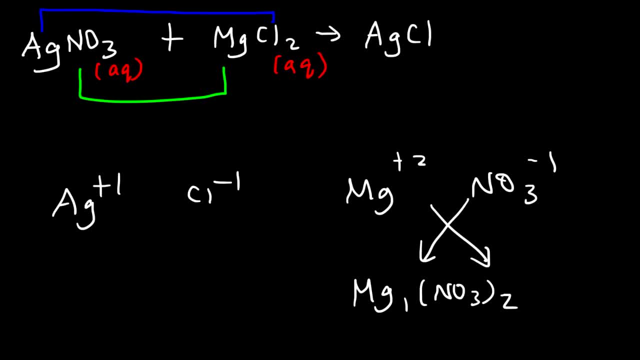 Whenever you have multiple polyatomic ions in a compound, you need to enclose it using parentheses. Now it turns out that nitrate is always soluble, so magnesium nitrate is still dissolved in the solution. However, silver chloride is insoluble, so it doesn't stay dissolved in the solution. 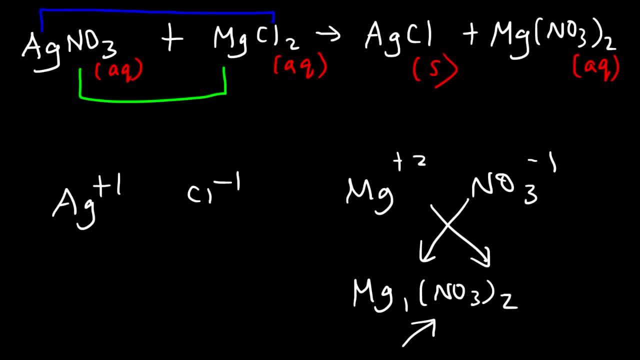 It's a solid product. Whenever you mix two aqueous solutions and if you get a solid product, this is not just called a double replacement reaction, It's also called a precipitation reaction Anytime you mix two aqueous solutions and if a solid comes out of it. 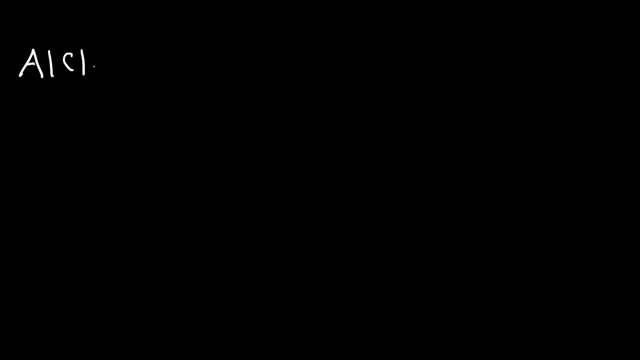 Now let's look at another example. What are the products in a reaction between aluminum chloride and sodium sulfate? Both of these are an aqueous solution, So feel free to pause the video If you want to try it out. Let's try this. 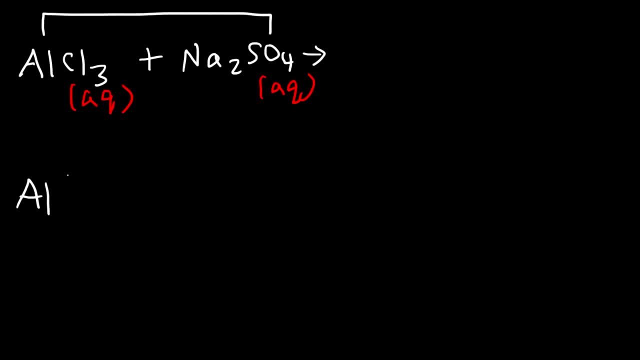 Aluminum is going to pair up with sulfate. Aluminum has a positive three charge, Sulfate has a negative two charge, So the chemical formula is going to be Al2SO43.. You just got to replace the charges with subscripts, So that's going to be one of the products. 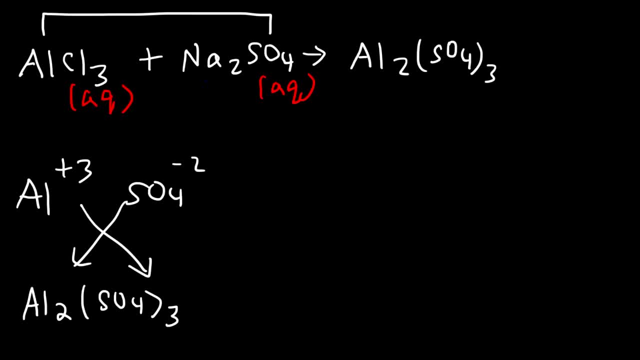 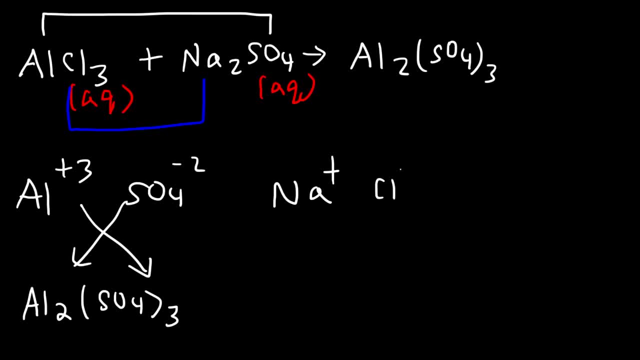 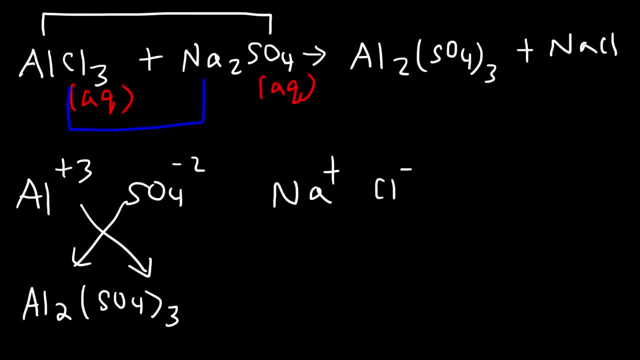 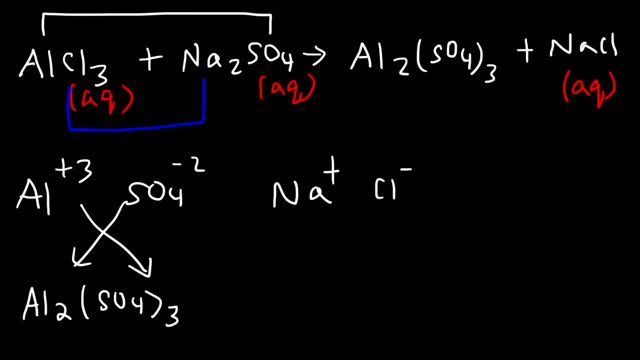 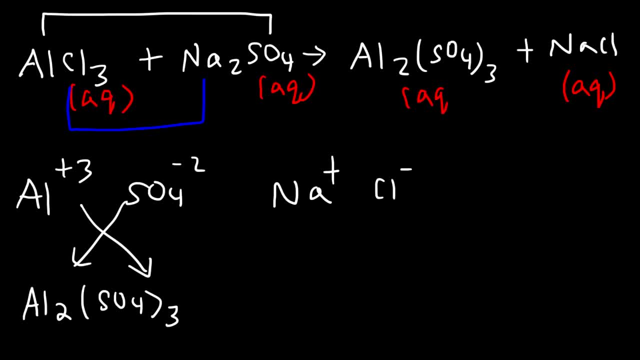 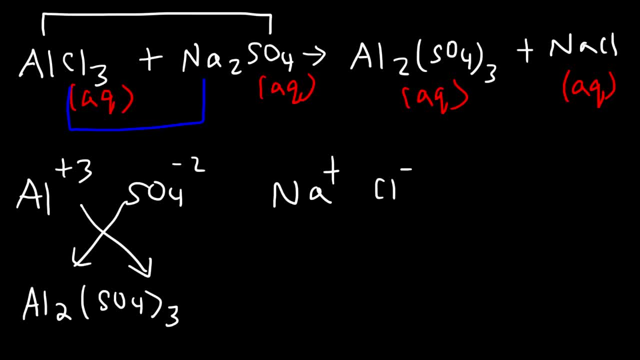 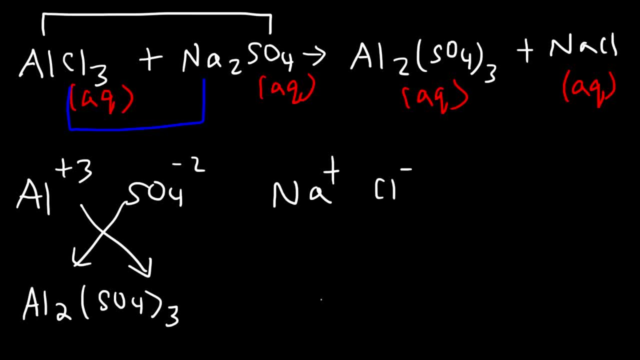 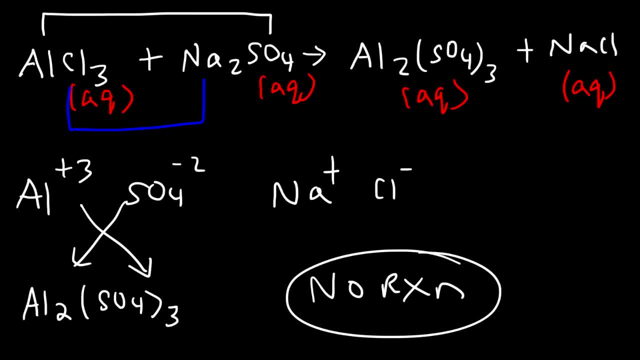 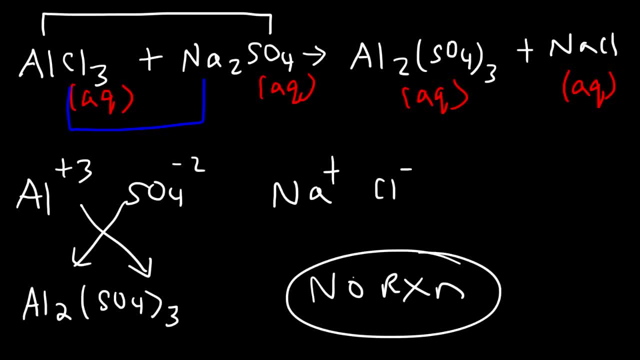 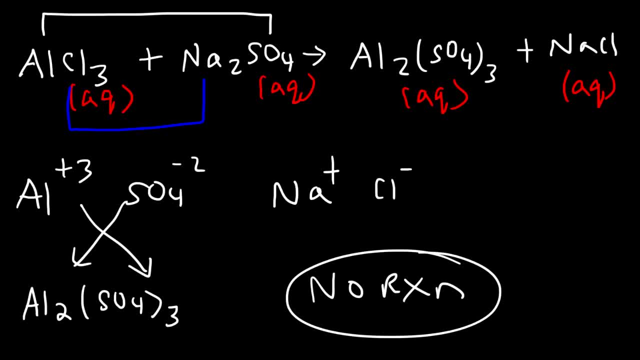 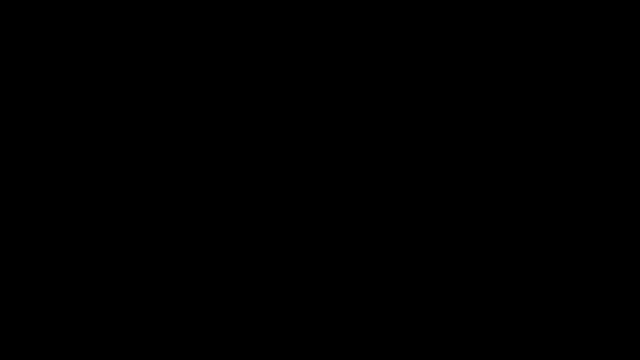 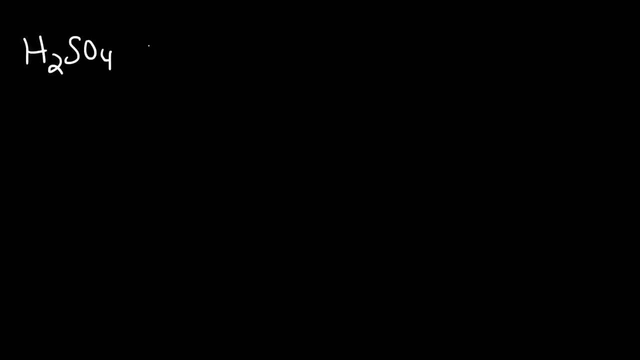 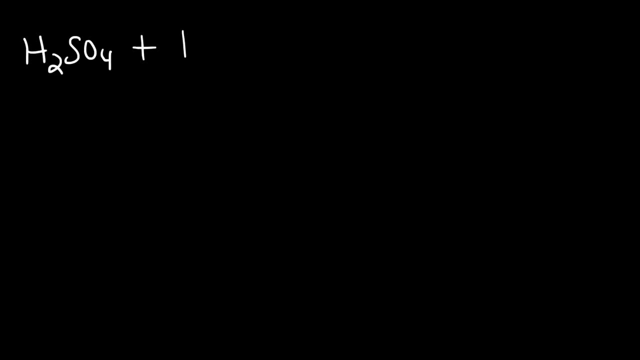 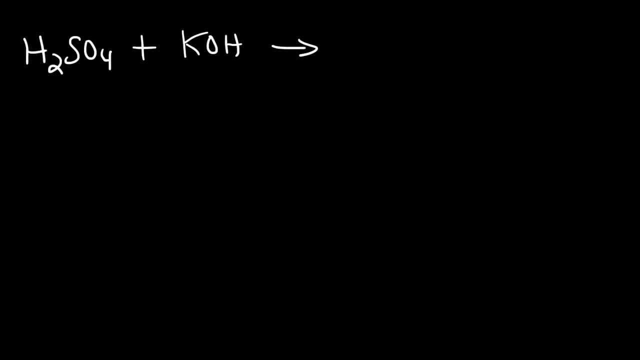 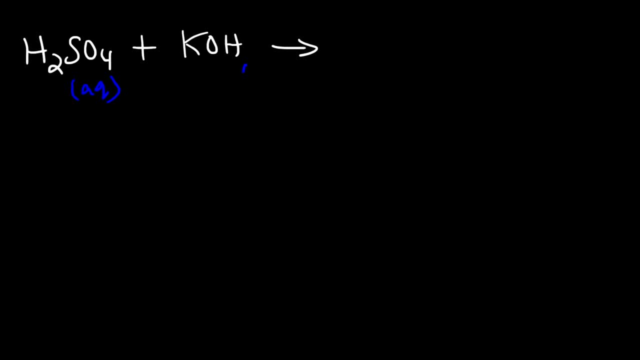 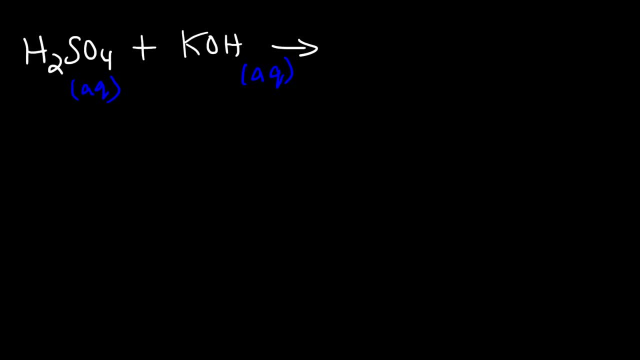 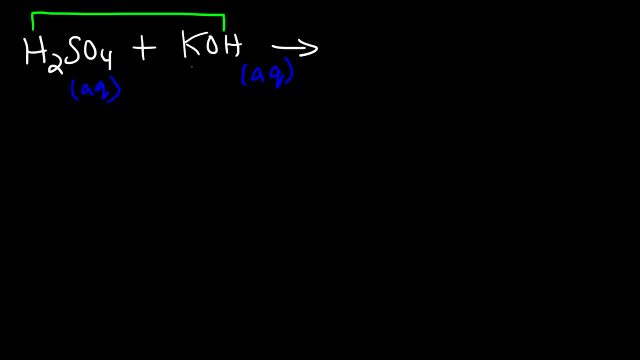 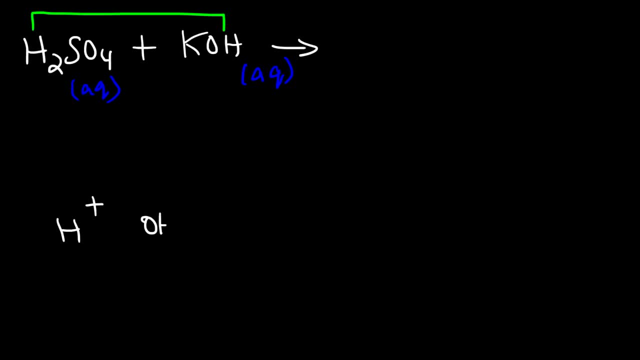 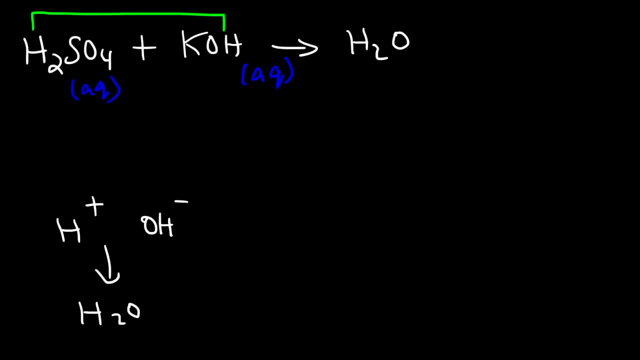 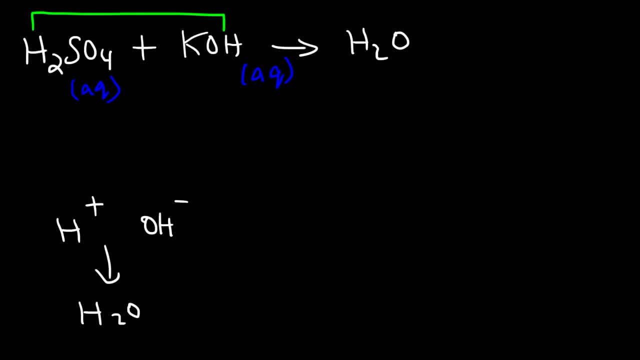 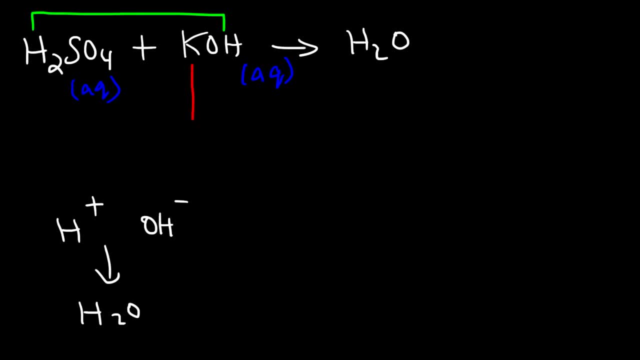 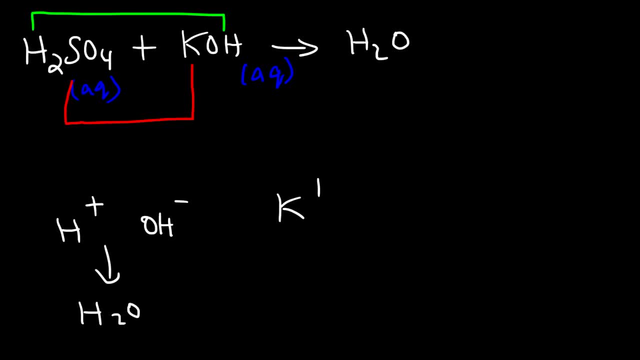 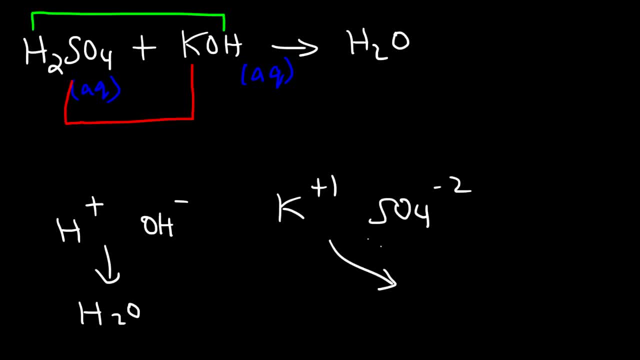 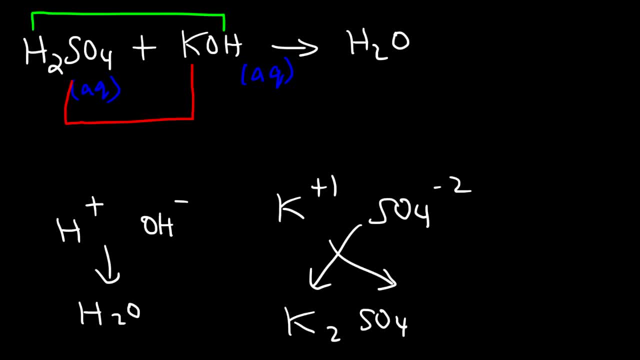 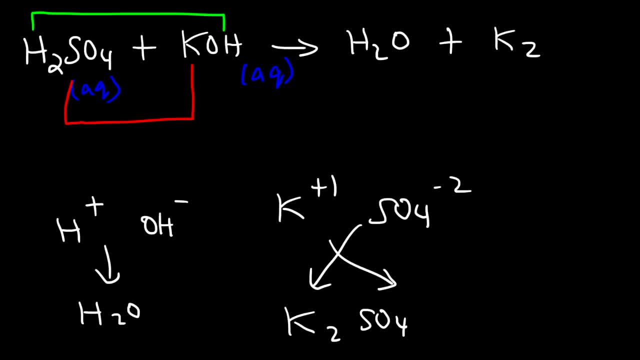 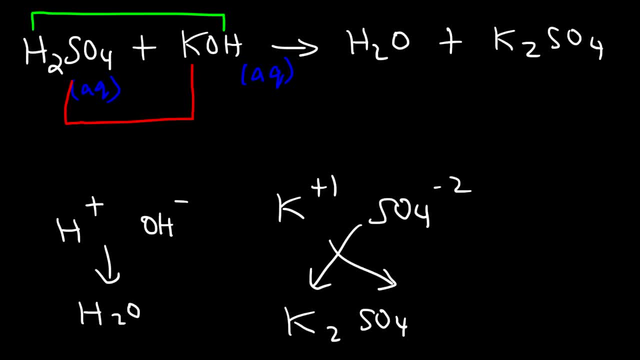 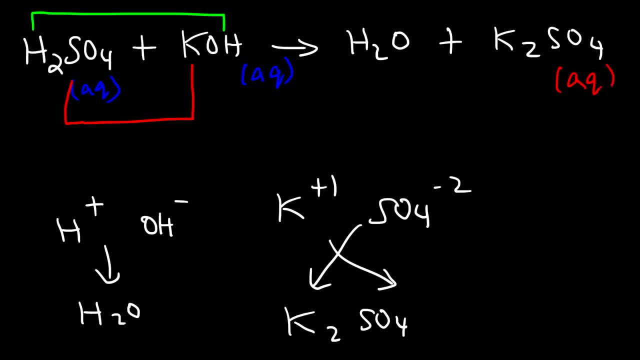 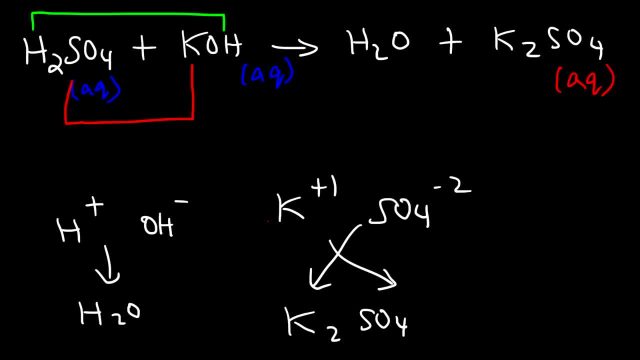 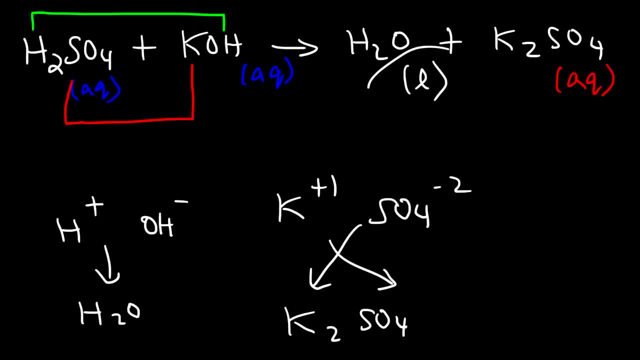 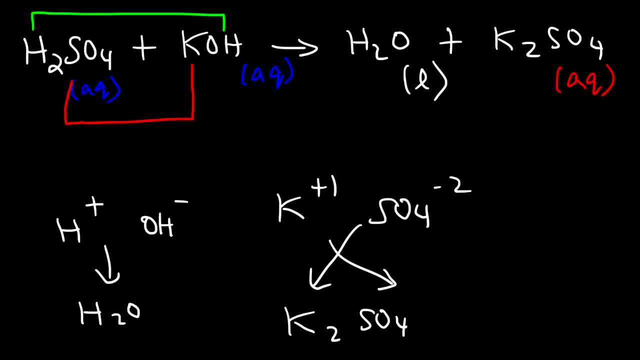 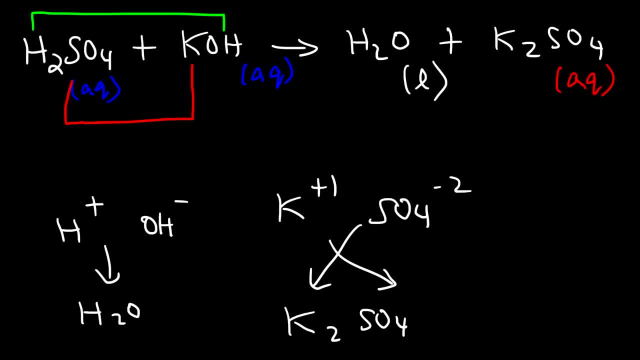 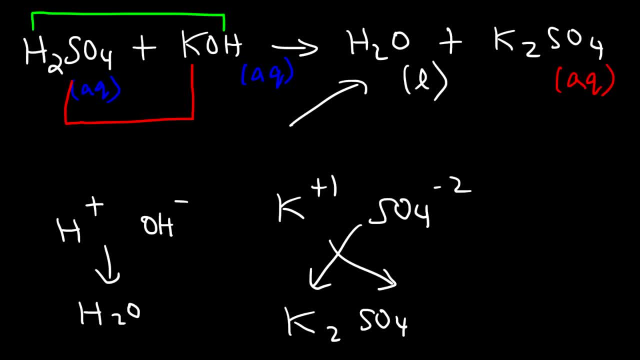 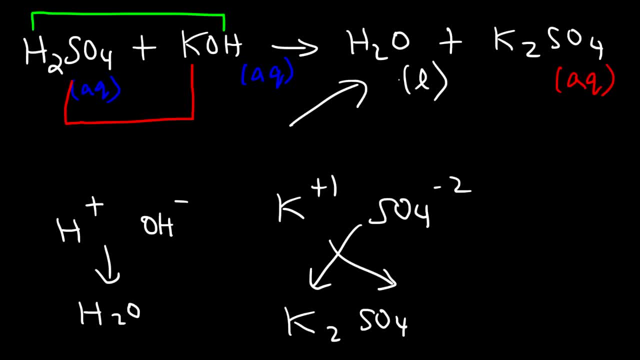 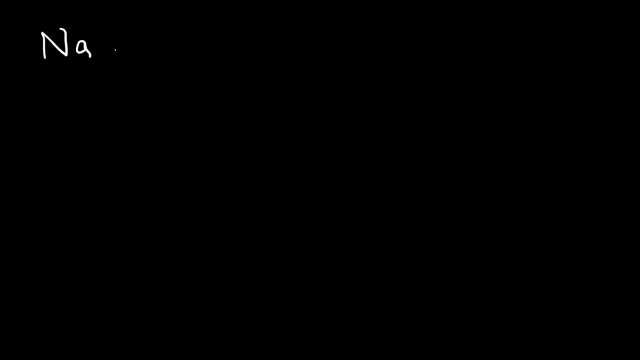 Let's try one more example. Let's try one more example. Let's mix sodium carbonate with hydrochloric acid. Sodium carbonate is going to be in the aqueous phase, and the same is true for Hcl. Go ahead and predict the products of this reaction. 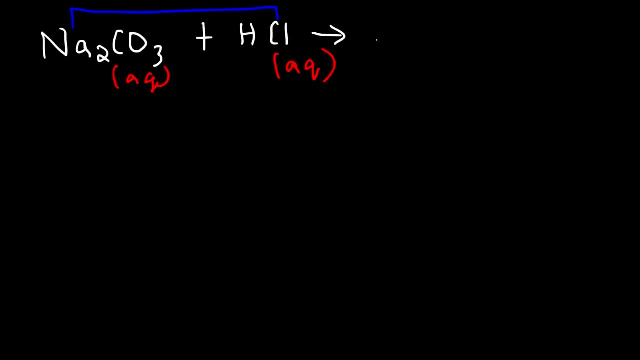 So first let's pair up Na and Cl, So that's just going to be sodium chloride, NaCl, And then hydrogen with carbonate. so hydrogen has a plus one charge, carbonate has a negative two charge. so initially, when you combine these two, you're going to get carbonic acid. however, carbonic acid usually doesn't stay like that at normal atmospheric pressure. it would stay in that form under high pressure, but at normal atmospheric pressure carbonic acid typically decomposes back into water and carbon dioxide. so therefore the products of this reaction are NaCl.